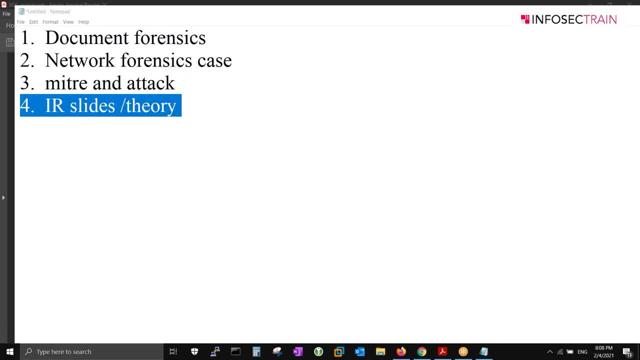 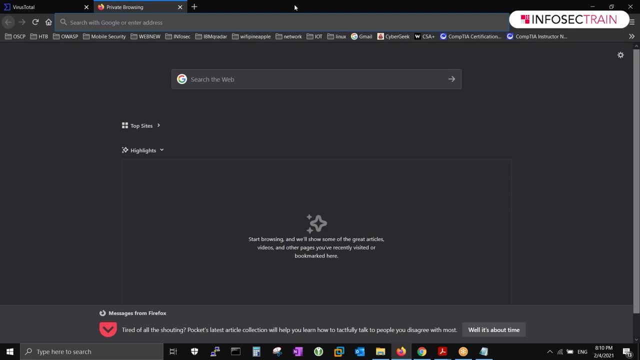 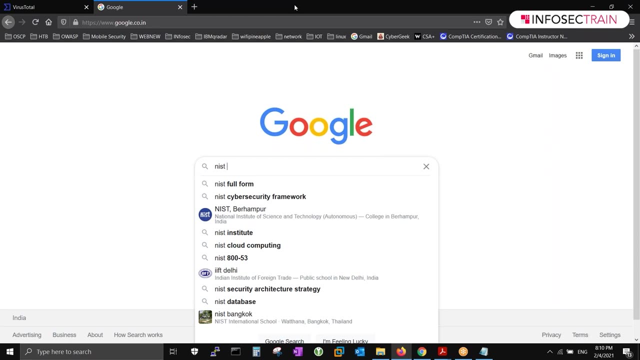 onto IR part. Okay. So, guys, there is a standard right now in organization. Every time we'll talk about standard part. Okay, Now see how same exactly what we studied. Same exactly This thing is there. NIST is their national Institute of standard and technology. 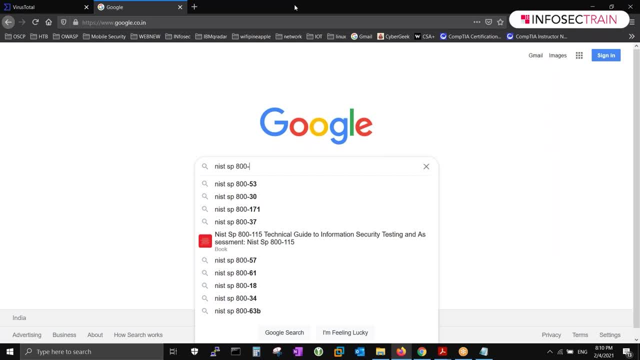 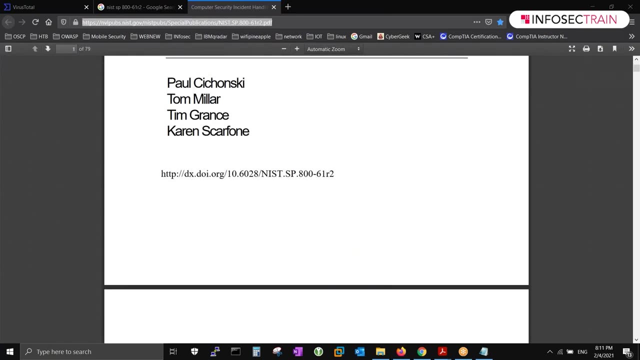 They have a special edition which is 861 R2.. R2 is released too. Okay, In organization, in companies. guys, we are following this incident response incident handling guide as per their standard. Have a look, everybody right. This looks like big Okay, So it has a couple of like policies. 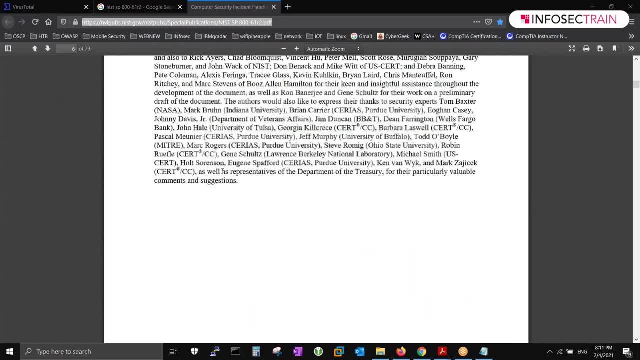 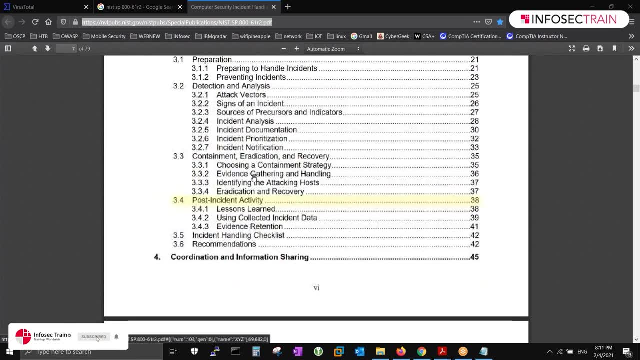 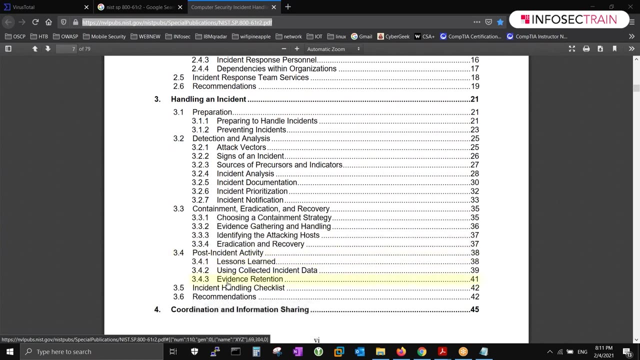 and all these things over here. right This, all things are there. You can see right now. they talk about policy plan, procedure, These things building up the team. How do we handle the incident in preparing, what we will do in detection, what we will do in containment, what we will do in post incident heart and what we will do? 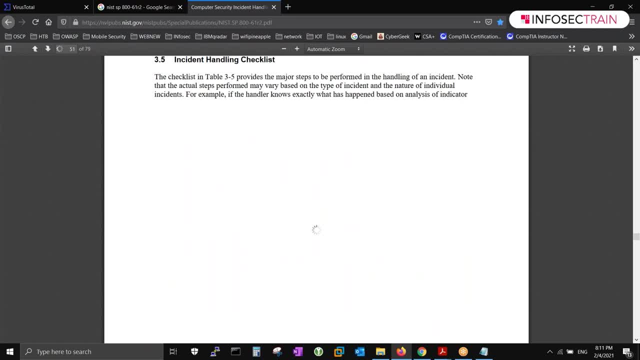 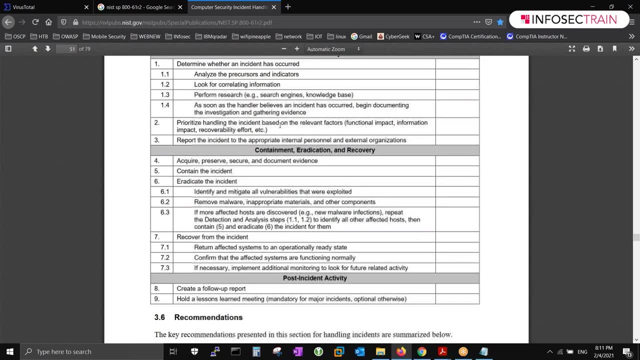 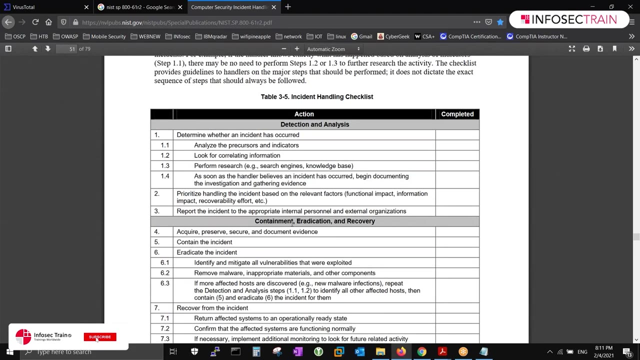 Okay, We'll be studying this thing. We'll be studying this thing through um, I would say through slides, and then I will come to this incident handling checklist. that what all things we should check whenever you are taking up the incident handling at your part over there. Okay, So no issues in that. 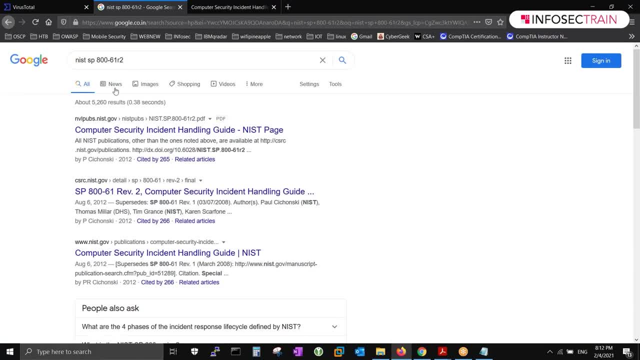 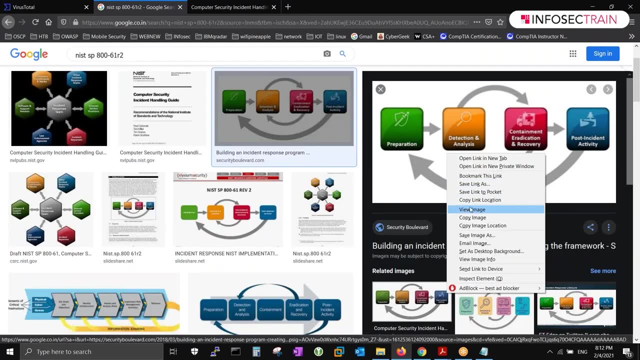 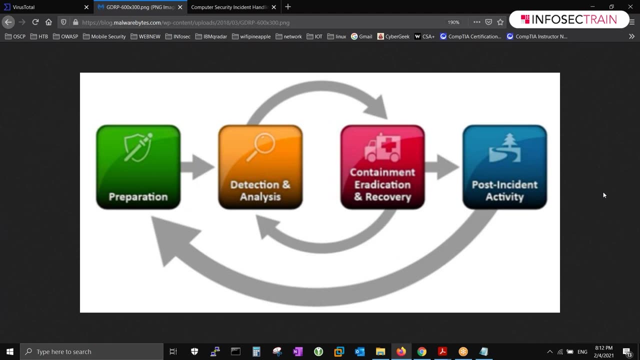 Cool. So first of all, let's let's talk about this. If you talk about the process, guys, it will look exactly like this: This is the exact process. image, Exact preparation, detection and analysis is nothing. but when you say like identification, this thing is there, Okay, And then you have containment. 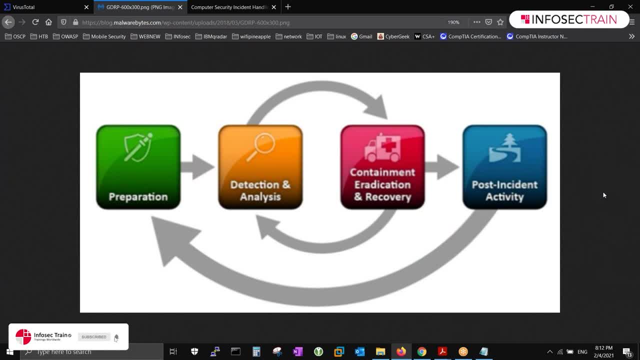 eradication and recovery and post incident activity- Cool, And you can see that it's an ongoing process. one by one, one by one. Everything is going on the screen. Okay, And really, to be very frank, it goes like this also Right now. 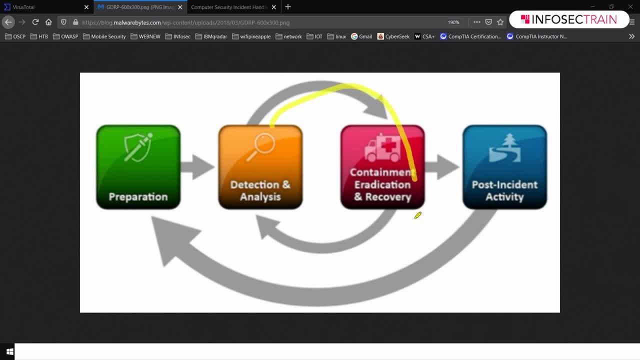 my only thing is: guys, there is like it is, you can say there is a circle, like it is going on, Process is going on And the last thing, it is a feedback loop. We call it, This is what we call. This is what we call. 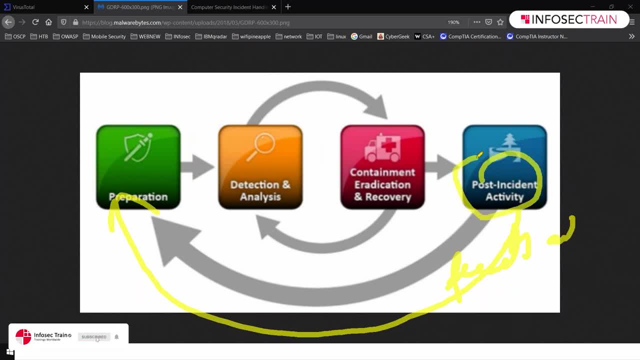 it as a feedback loop. Okay, So after post incident activity, why it is again going to the preparation stage? See, guys, after the incident, what happened? knowledge base is fine. Okay, Knowledge base is fine, There is no issue. right, See what we are doing is we are doing a? 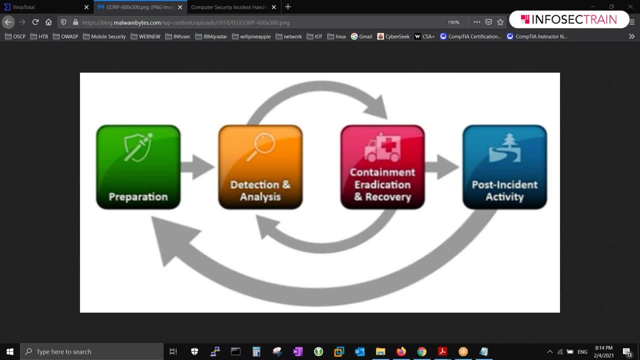 re verification over here So you can say current, after recovery, we'll do detection analysis again. Okay, No, like it is like you close the case sometime happen after a couple of period of time. It can come again. You need to like prepare for it next time also, Right? So let's suppose you are like. 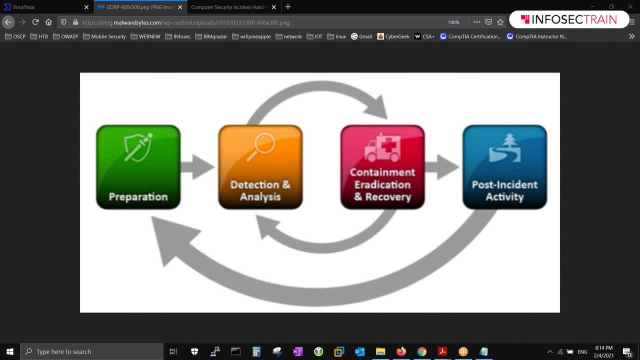 signature based thing. You talk about ransomware stuff. You talk about emoted thing, Trojan malware, anything you talk about That have a signature, that have a pattern. right now, what we do is, after that it will go hit and it will. 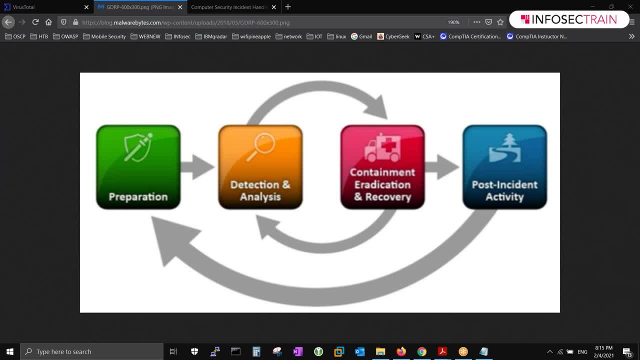 again recur in the environment. So we have to like prepare with the new stuff. Maybe it will change the signature, Maybe it will change something else, but you have a reference. So, as said by Mr Grady, you have a reference right Already in the lesson run. in the run books We write everything over. 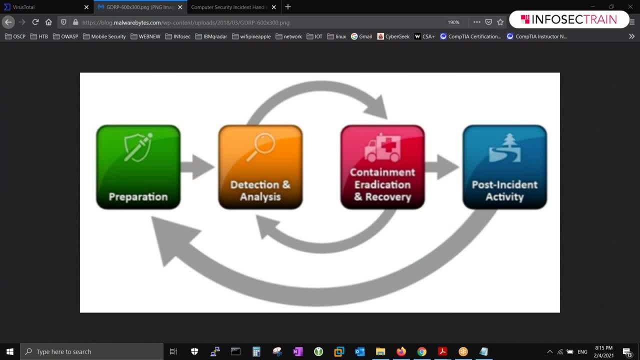 there. Okay, So there's the reason we are going over this and this, this four stage thing. right, Because yesterday we studied preparation, identification, containment, eradication, recovery and then post-incident activity, or like lesson learning. So over here it is concise to four missed SP 861 standard release to 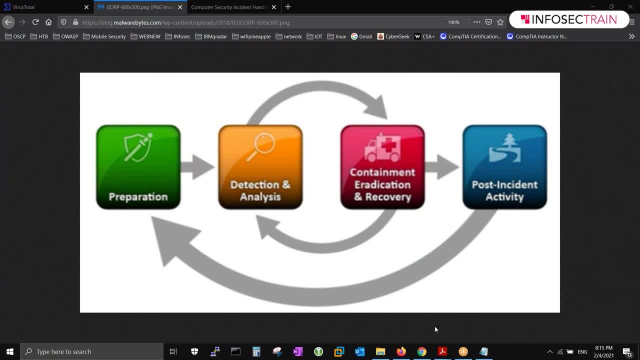 standard. It is using this thing only over there, right? Is that clear? Now I'm going to, one by one, again revise with you that. what happened exactly in preparation? What exactly happened in containment, eradication, post-incident and detection, right? 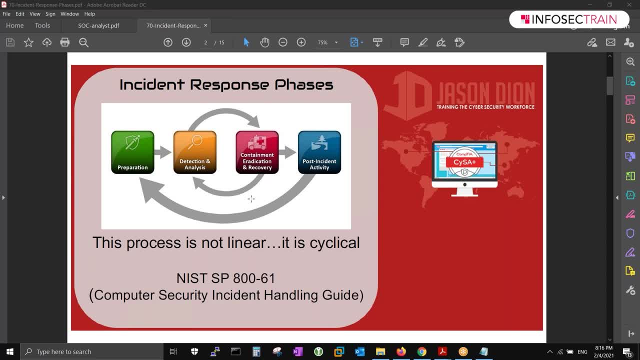 One I want to see over the screen. This process is not linear, This is a cylindrical process. That's the reason I ask you that feedback loop. Okay next, SP 861 is in standard, National Institute of style, standard and technology. SP is spatial. 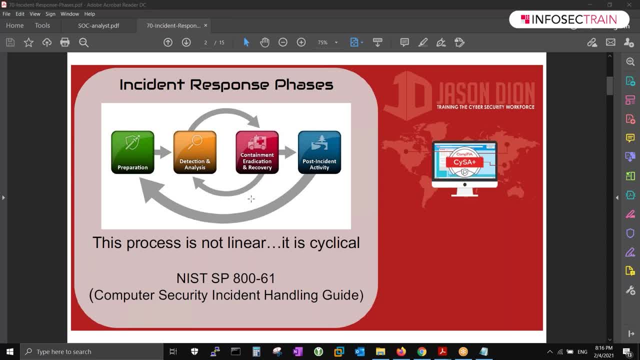 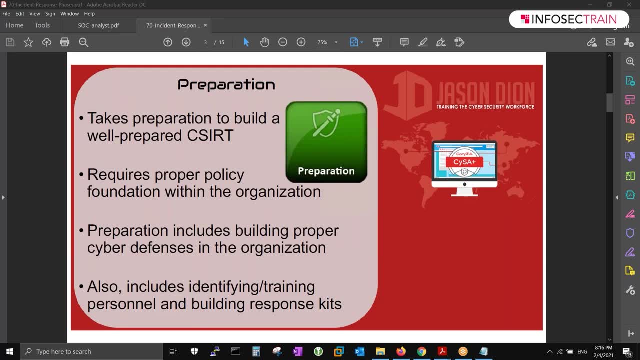 publication 861, release R2.. We are using in the industry standard. Okay. second thing will go one by one. yesterday We talked about that If you will build up a team, hundred percent right will build up the policies. So P right, you talk about scope of work, what we need to do, right. 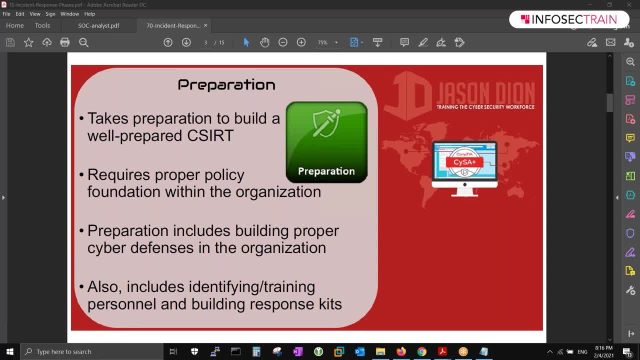 So here I would say now something add-on we will see up over here. preparation includes building proper cyber defenses in your organization. to be very Frank, to be very Frank here, We can talk about security trainings Also he can. we can talk about, like training up a personal on a particular product. 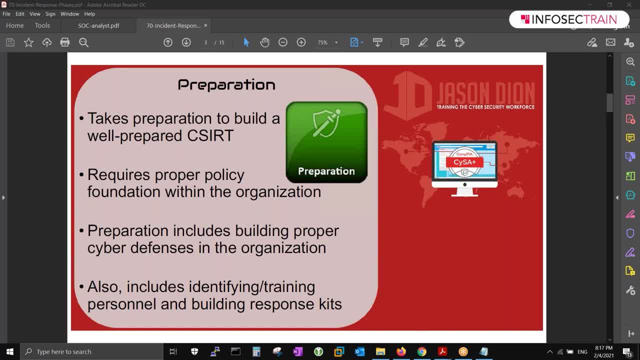 Let's suppose you deploy a email gateway. Let's suppose you deploy- maybe you can deploy- something like 40 net firewall, Is there? okay, We can deploy that to. let's suppose you deploy a UTM solution, FireEye solution, Okay. so these are some products in the cyber security- good, costly product, and we are going to give them training. 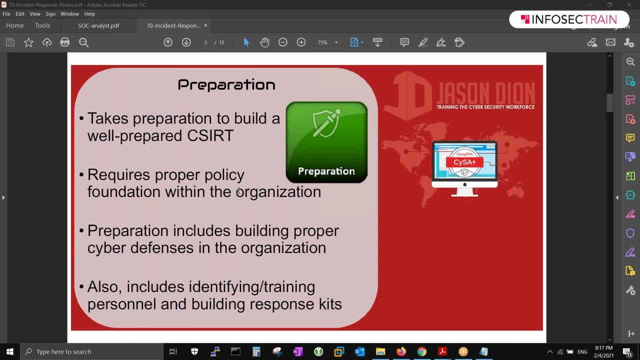 that is also coming in the preparatory stage. You're making your cyber defense strong over there. Okay, policy procedure, these things will come over here, No problem. building up the cyber incident response kit? Okay, that is one of the stuff. what, all things, we will include? 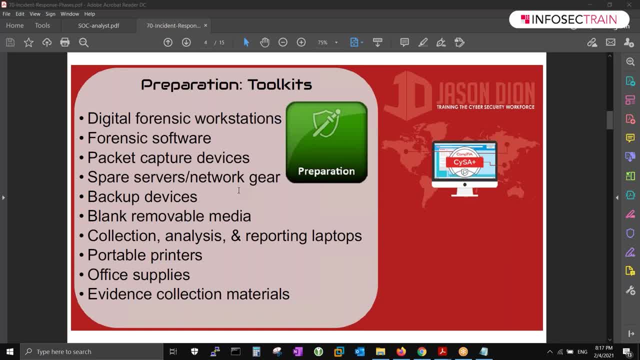 See over here: digital forensics, workstation forensics, software packet capturing devices, spare server, network gear for this kind of stuff. at any point of time You want to go for a remote investigation, You can go. backup devices, portable printer, all these things, evidence collection materials, these things you require. 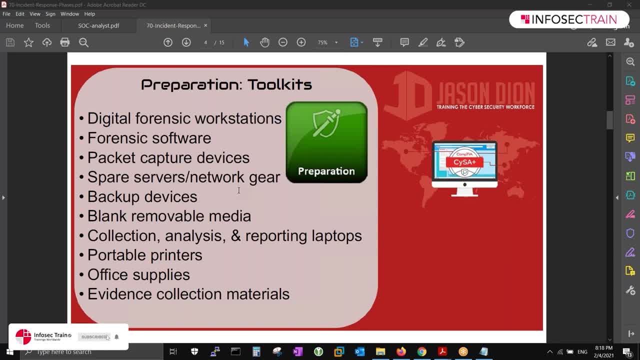 I'm not saying like we are doing a human investigation over here, We are doing a digital investigation, Okay, so all these things are required to be very Frank. So, basically, when you're talking, Talk about CSI, RT, that is, computer security incident response team. 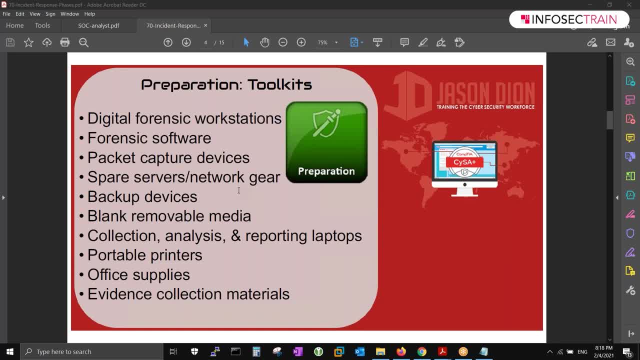 So whenever we are talking about this term, we are mostly talking about tools that are, like I would say, portable. I would say that are that can be run on a live environment easily. you attach and you can run. there is no extra things You should require to run it. 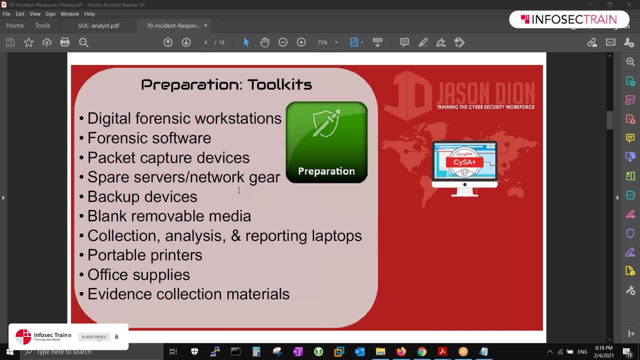 Okay, so live, things are very much powerful over there. You go plug and play and your device work starts working over there. These kind of things we require, Just like we talk about your thread server. red server works on ports Mostly. you have a hard disk. 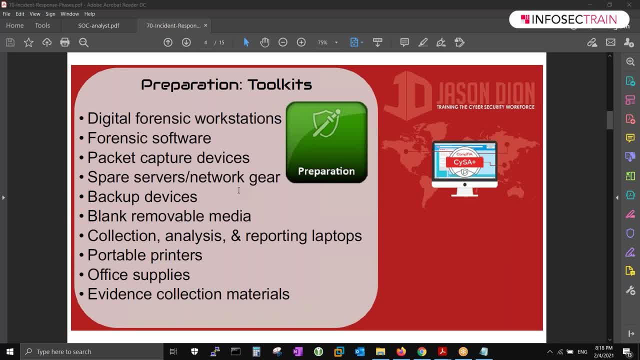 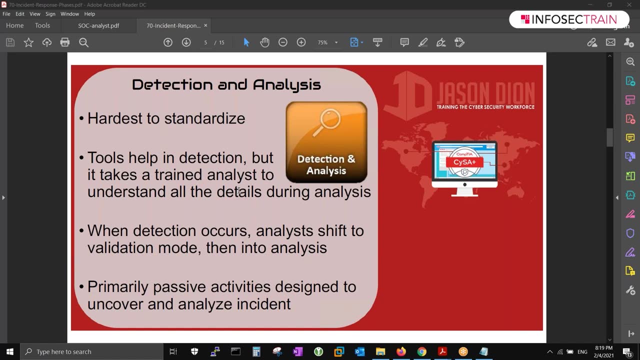 Okay, just swap the hard disk over there, Put it in the disk system. You're good to go, All right. So these kind of fast things we require over there, Cool, Perfect. Then if we talk about detection and analysis here, we will be discussing about yesterday, guys, that how will you do detection and analysis? 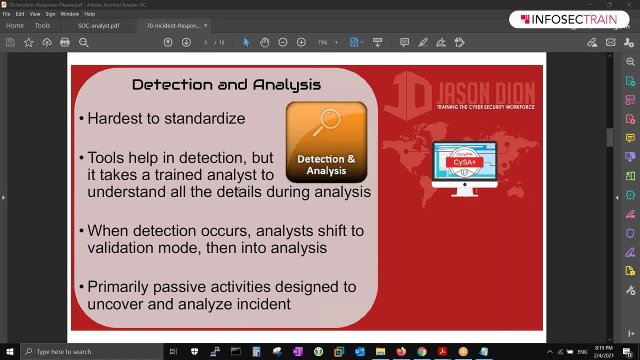 So we talked about like: we have some solution, We have tools, tools. We have fingerprint detection. There are now more tools coming up in the market, guys: UTM is there, Firewall is there, IDS, IPS and AI is already being started inside. I am talking about artificial intelligence. 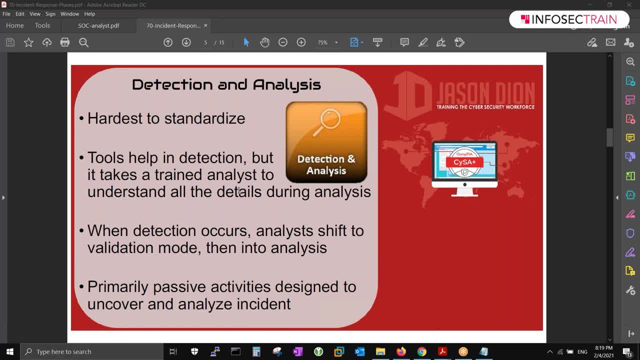 They are so much smart right now that they will do half of the work themselves. There are so much fine-tuned, I would say right now. Okay, so you can say like passive, primarily passive, activities designed to uncover and analyze the incident, Primarily. 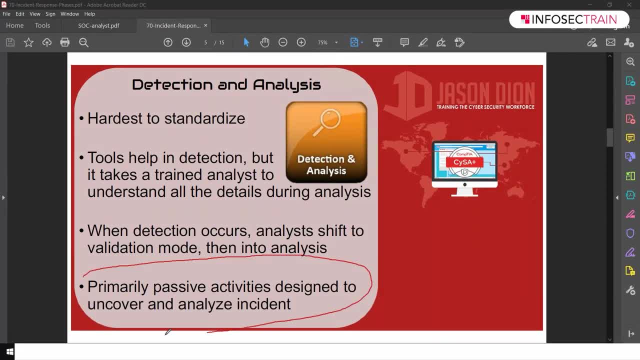 Okay. So last point is quite impressive over here. What is a passive activity? over here They are saying passive activities are designed to uncover and analyze the incident primarily. What is the meaning? So you can stop from the real-time monitoring. Sim solution is there. 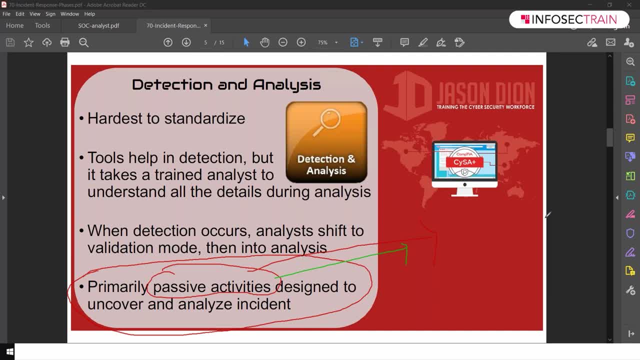 You can stop from there also, right? passive activity is something, guys, If you remember, like if I give you a PK file, that is nothing but a passive analysis you are doing up over there, right? So primarily, I would say why they are writing this thing. 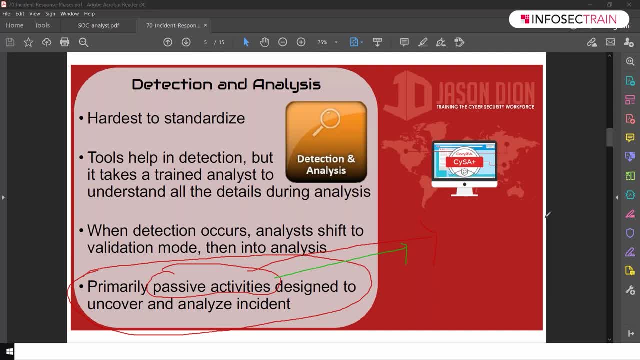 Most of the time, you will get to know that this has already happened. now, right, I'm taking the future thing, which has already happened. Now, That's why they call it that this kind of incident has happened with us. real-time incidents are there. 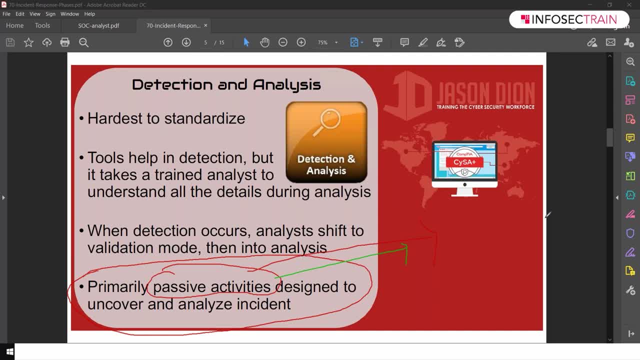 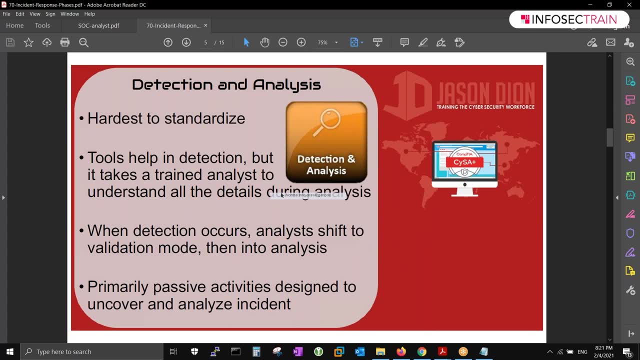 I'm not denying, but most of the time they are. you get to know after it has been done. There's the reason it is written like this: Okay, cool, Let's proceed further. They talk about alerts, logs, publicly available information, people, right. 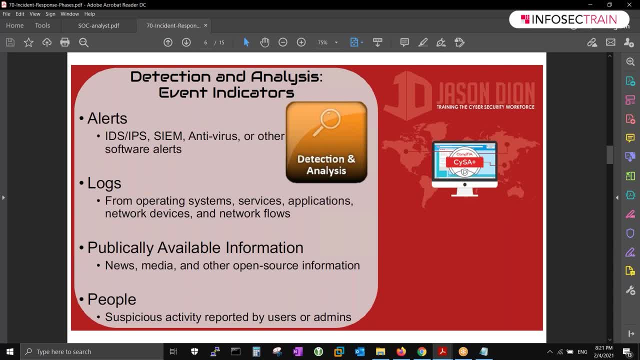 So alerts, alerts coming from, you can say IDS, IPS, intrusion detection system, intrusion prevention system, same solution and other software alerts logs. We have seen guys, We have seen your Windows logs, Linux logs. You can get your network logs Also, network device logs. 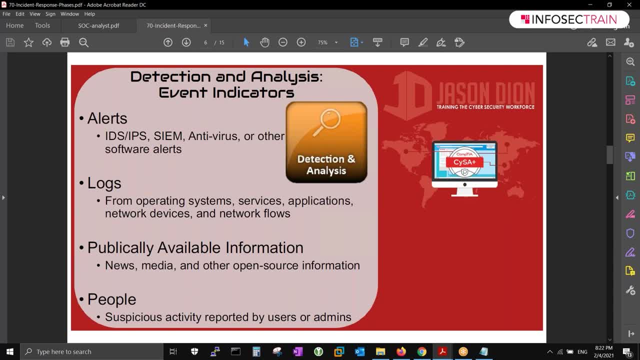 Also application log, also any log you can get, okay, publicly available information. yesterday We took an example of that, that how to find email of a corporate good to go easily. You can find cool. if I give you a number, Let's suppose I give you a. 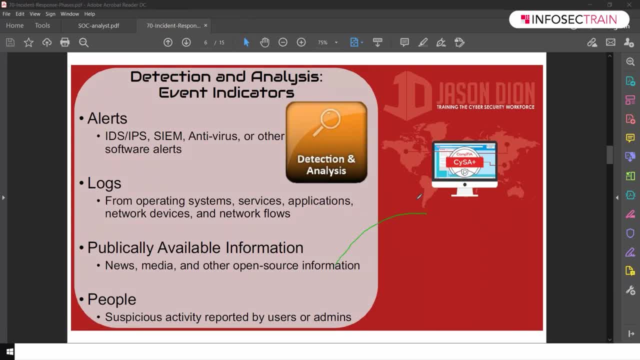 Number right? So, guys, if I give you a telephone number where you will search for it- Totally ocean time talking about- if I give you a phone number where you can search information about that number, Will you check in your social medias or not? 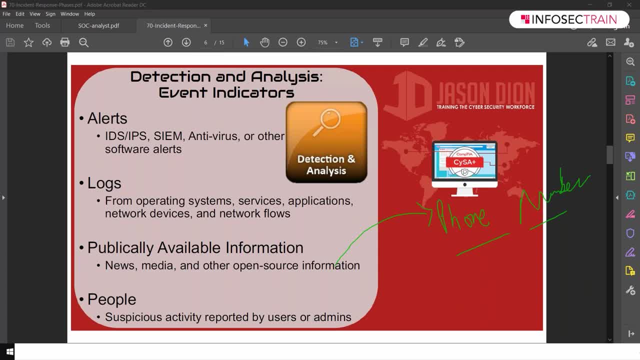 You will check for sure, hundred percent, right. Right, Don't forget, guys, telegram and Skype. Don't forget these areas also. Okay, you will get some good information over there as well, because people are using these kind of stuff today. All right, we'll be talking about OSINT, will be talking. 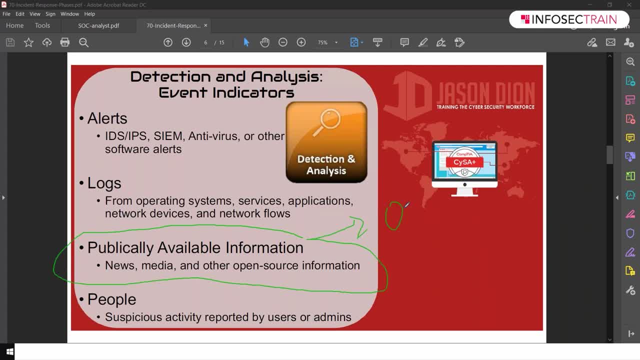 This is completely like OSINT. We call it open source intelligence. OSINT is there. Okay, we'll be discussing this thing when we touch threat intelligence part with you. then you will get up to know all of these stuff. Okay, people, you will get information from people as well. 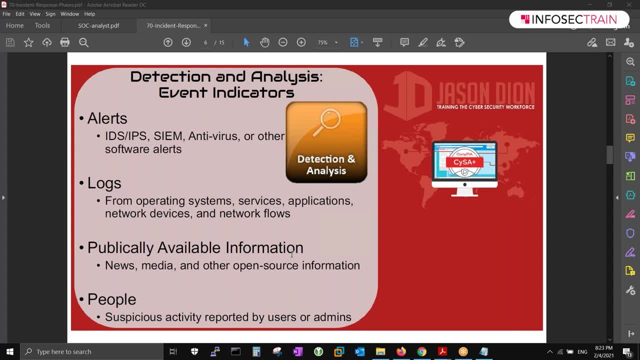 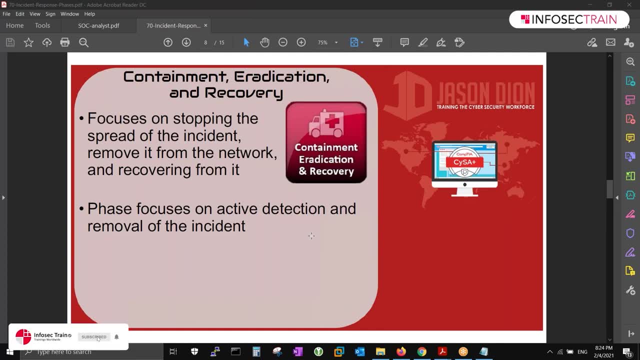 There is no problem in that. Okay, then we'll talk about, like your, containment, eradication and recovery. So containment, eradication, recovery is nothing. There's a proper five steps are there? I'm going to discuss you Five steps. meaning remains the same. 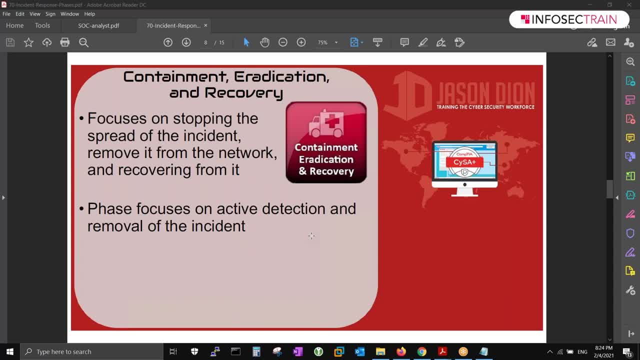 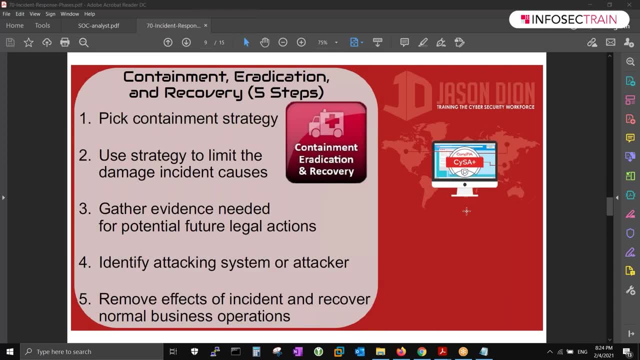 You can see, focus on stopping and spreading the incident, remove from the network, recover from it- simple, simple right. But there are like five steps you can see over here similar. They are taking pick containment strategy. Okay, So when we talk about this first point, they're writing containment strategy. 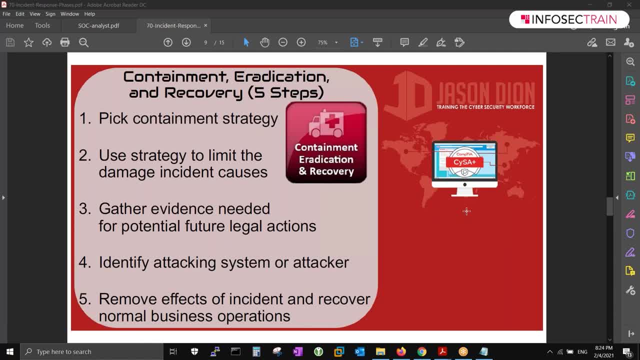 Like I told you, like critical server is over there, Okay, and we are talking about intacting that critical server, or you want to give the uptime to it, Okay. Now there are possibilities. certain situations are there where you're not able to inform to your customer. 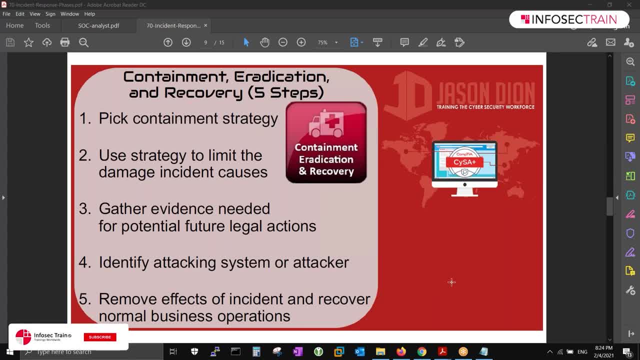 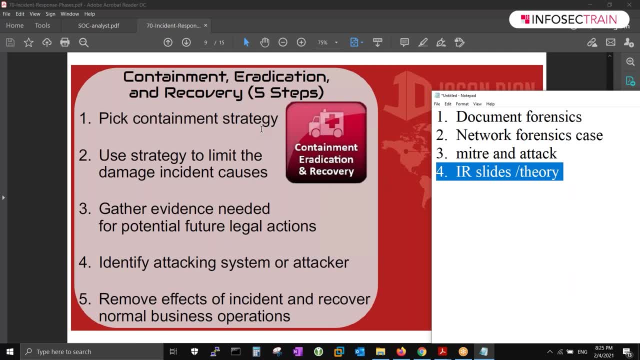 to your member form that this thing is happening with us. cool. in that manner, What will happen? that you have to like, accept and you need to close down your certain services, like yesterday, We were talking about cluster, So one cluster is up, then another cluster is closed. 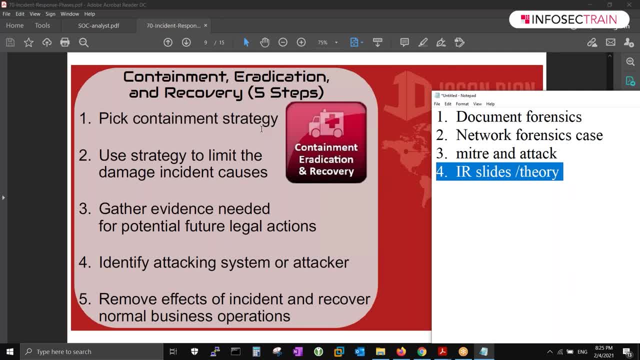 You will fix that and make it high availability over there. We call it H a high Availability over there. Okay, so possibilities there, we can talk about that as well. use the strategy to limit down the damage and the incident causes. most of the time, guys, most of the time. 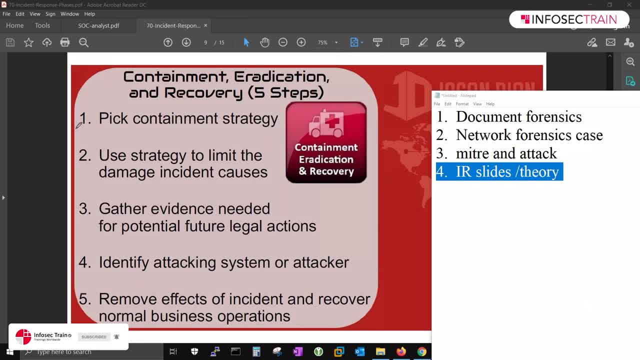 Let me take an example over here. So, guys, let's suppose there is a huge request coming to one server, huge DDoS is coming. Those are DDoS distributor, distributed denial of service or denial of services coming. huge request is coming to you. 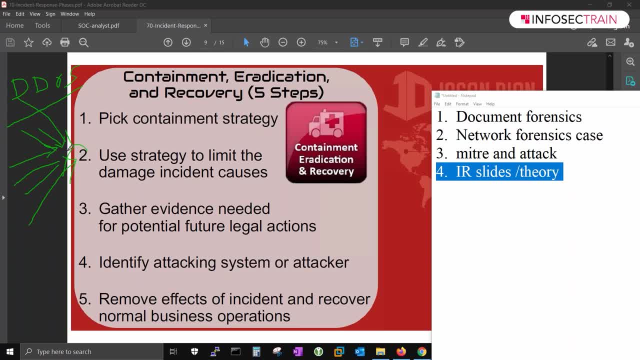 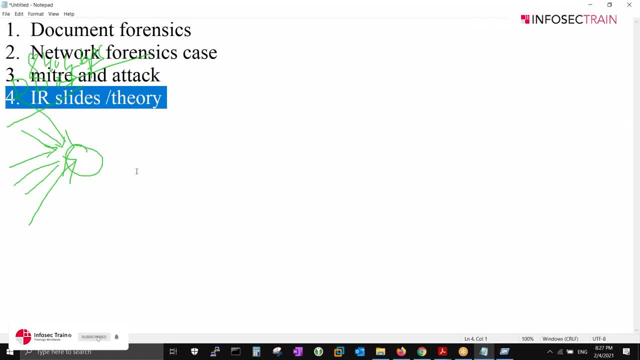 Okay, What is the best strategy that you will apply on a particular server? Anyone heard of sinkhole? What is that? Diverting the traffic, hundred percent, right. So see over here, guys, what will happen. This is there. Okay, what we'll do. we will like redirect the traffic to where we call it like a DNS sinkhole. 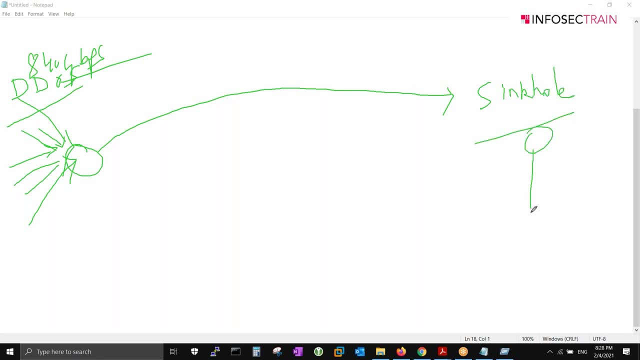 It's a place where you will like reach up the packet over there and you will start dropping the packet over here If, if the Nature's or the validity of that packet is not matching with your infrastructure, right. So acknowledgement packet is like it is, a there is a time limit. 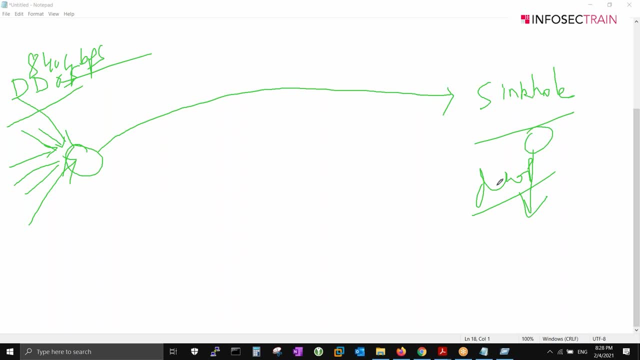 We can hold now so that you can drop, start dropping that part. another thing which people play over here Also: you can play about your network load balancers over. also over here. You put LBD and you do like sharing between the network load balancer and you can minimize the risk, I would say, or you can. 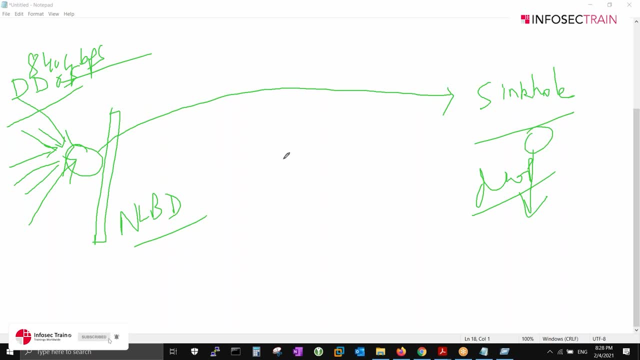 let's suppose 840 gbps. It will disperse into the network load balancer, but 840 gbps is actually huge. It will come from a cloud traffic. Okay, so it's not like one mitigation. You have to provide multiple things over here, sinkhole. 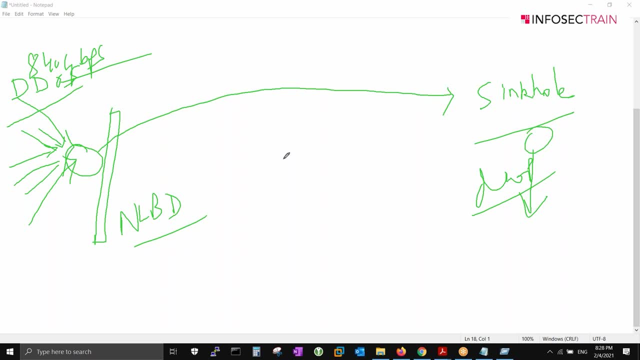 You can use, and LBD you can use network load balancers over here and, like you can use in clusters to be very different, different instances, So they will disperse the traffic. so it will be like I would say it will be dispersed into three or four. 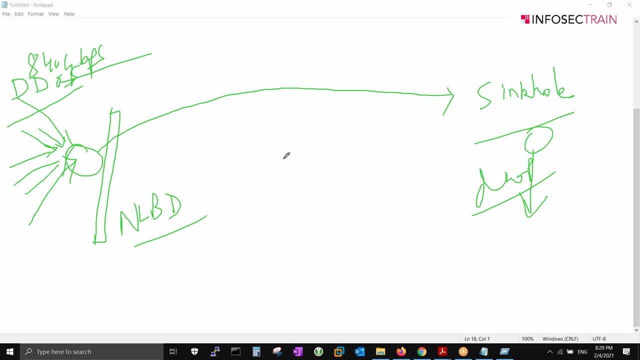 Network balancers and it will suppress the attack that is coming to you. Okay, anybody can play up with the game also, like they generally come up with multiple source ips. Okay, multiple source ips, they can play over there also. cool, Sometime they come up with the like a volumetric attack. 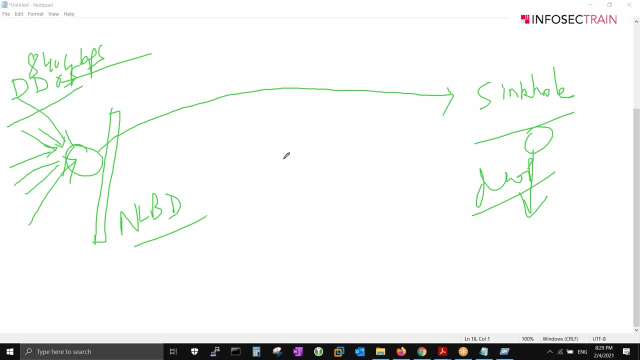 They will just come and they will just start bombarding over there. Sometime they will come with a very silent feature. It will come with a small file and then they start eating your resources Into your system. Possibilities there, small file that taking into your resource system. 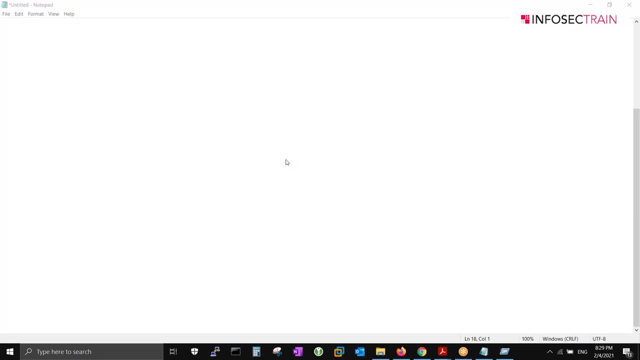 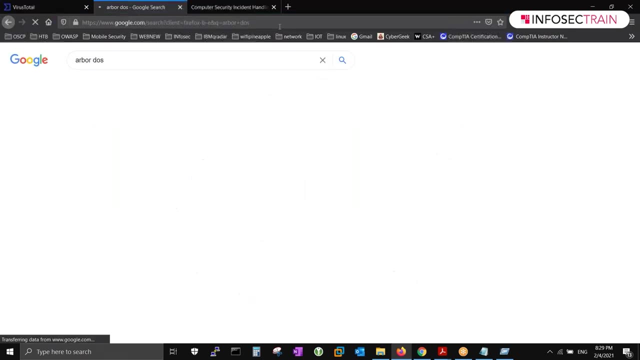 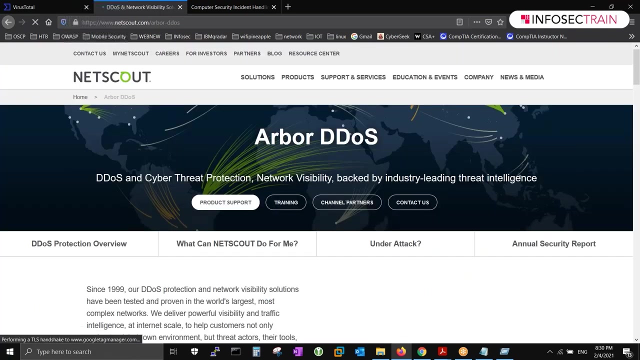 Okay, possibilities there in order to remove it. guys, We have a lot of protection stuff in the market. One of the best that almost every corporate uses up is Arbor. Okay, Arbor is a very nice tool in case of TDoS protection. interesting tool over there. 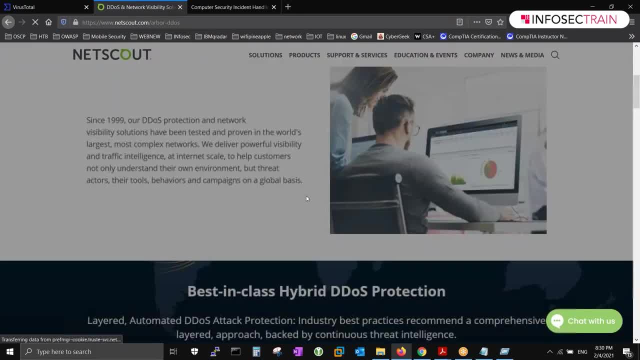 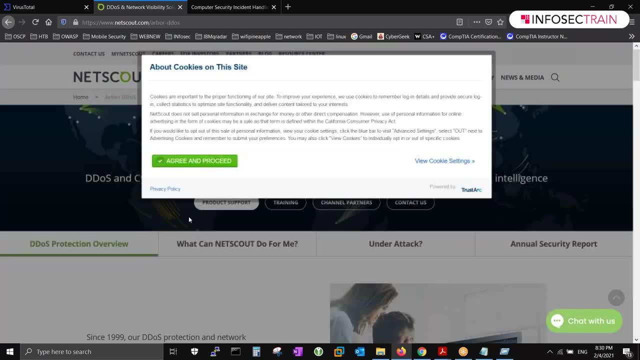 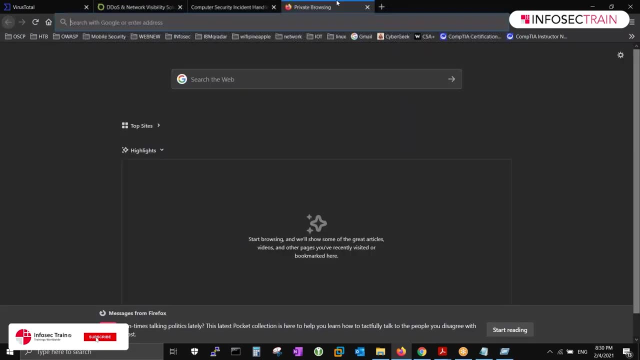 Right, interesting appliance. I can say It's a complete. the dashboard and the working layer on all the OSI layer is. it's very amazing, Very amazing. tool itself is very amazing. The response is very good out there. Okay, second thing, which most of the fortune 500 has also implementing: that is nothing but your watch guard tool. 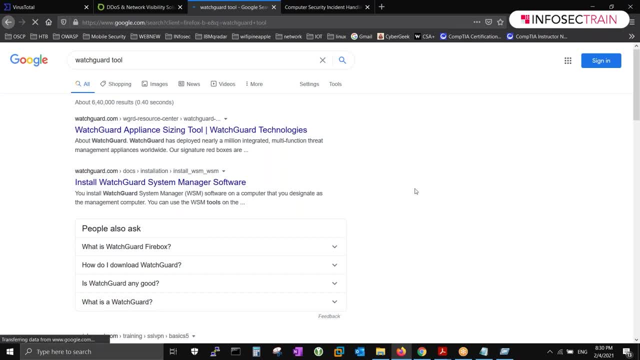 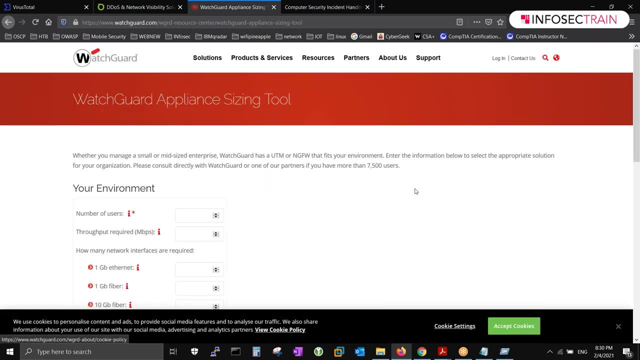 It's all commercial. Okay, it's all commercial. watch guard is also good for your network security. Very good product. I'll showcase You both of them. this one also watch guard- Okay, especially just for network security. This thing is a very amazing product. 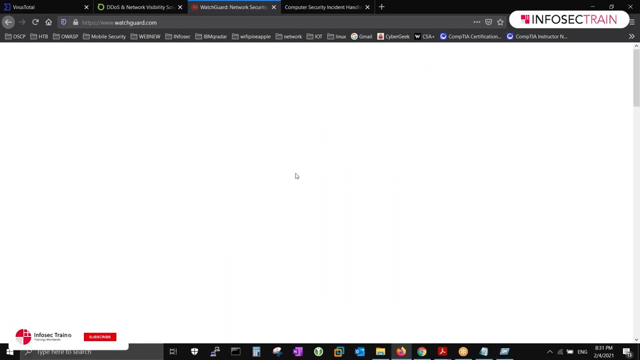 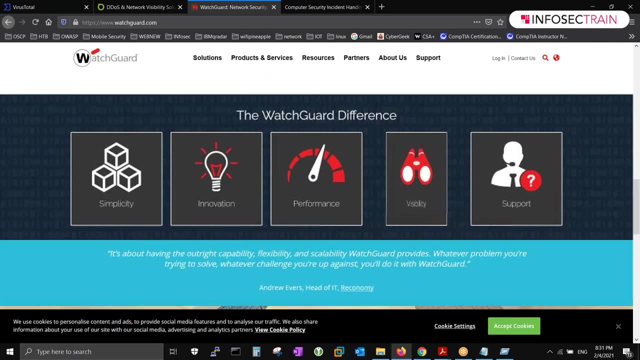 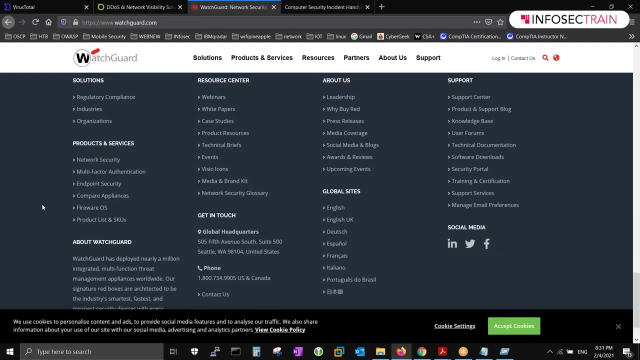 Very amazing product. It will safeguard you from lot of network attacks. Lot of network attacks. Zero, zero out, Samuel. all this thing comes up very nicely in through web. Okay, it will guard you in a very nice manner over there and it follows very much good compliance. 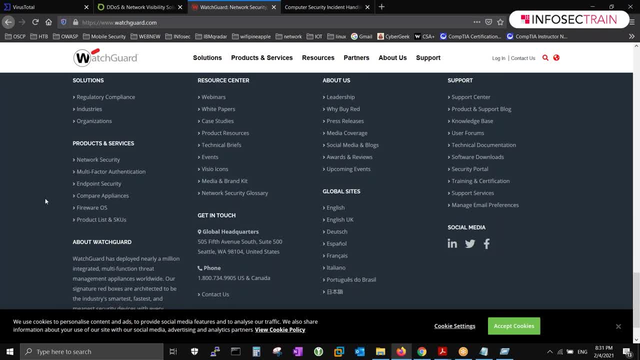 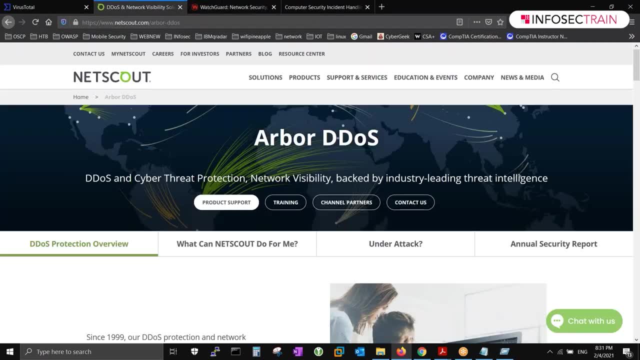 Also PCI, DSS, HIPAA, all those common things socks You talk about. they follow all those compliance rules as well over there. Okay, so these two things you can keep it with you. At least you should know about them that these kind of things are there.